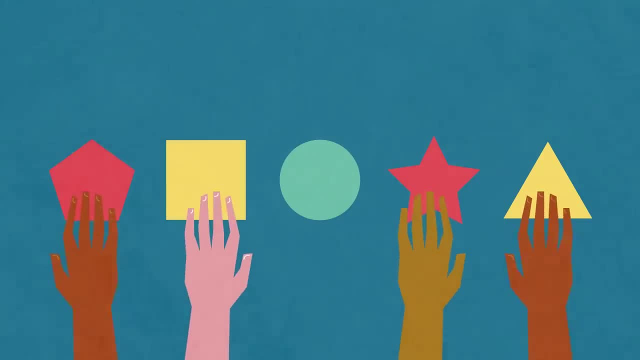 is a way of thinking. It's recognizing that all of our students bring different gifts and challenges is one way we might differentiate, like allowing students to choose their research topics or essay prompts. As teachers, we need to keep our eyes on the prize. In other words, we have to keep asking. 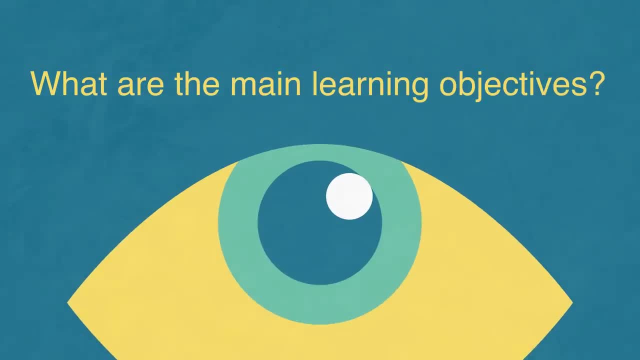 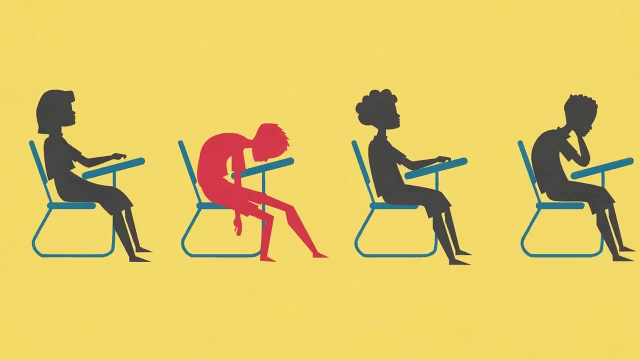 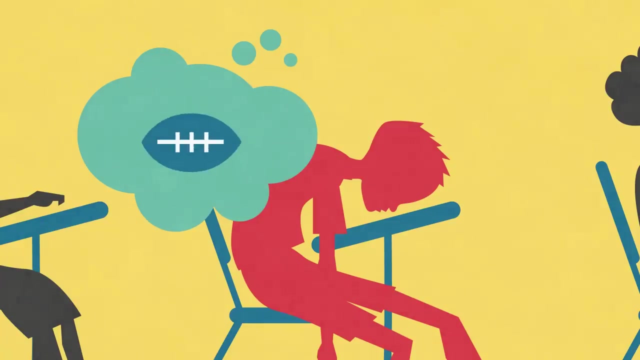 ourselves. what are the main learning objectives? One day my students were writing an argument essay about what would be the worst natural disaster to experience, John's head was down the desk. He was not doing anything. I knew that he was interested in football, so I told him that he could write an. 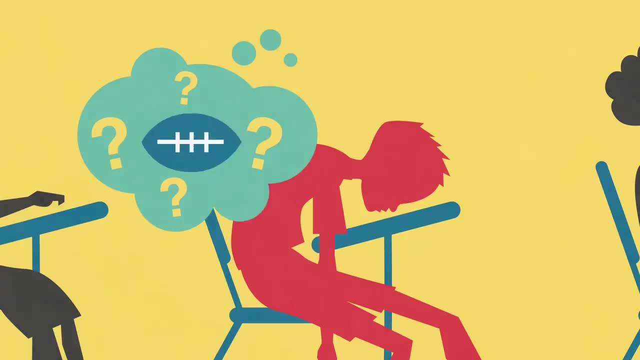 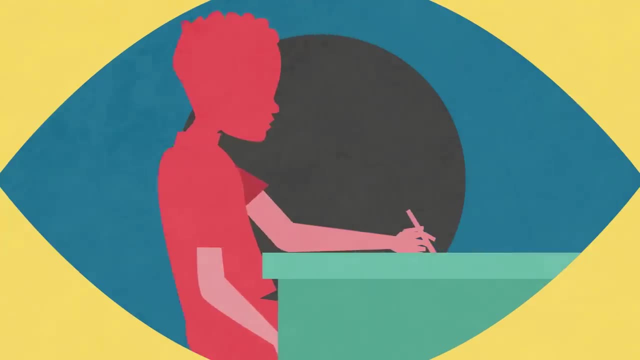 essay on why his favorite team was the best. He would still have to make an argument just about football instead of hurricanes or earthquakes. His eyes lit up, He got to work and wrote what his mother later told me was the first essay he had ever written. in school He had followed all. 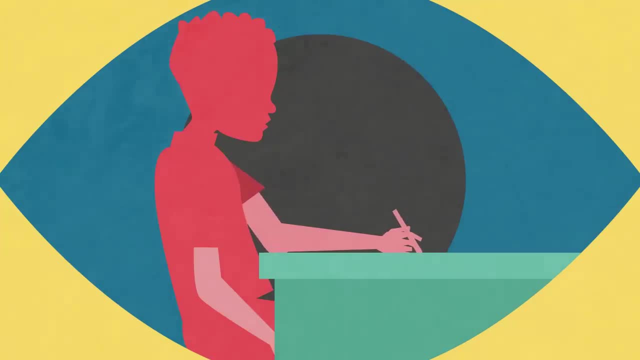 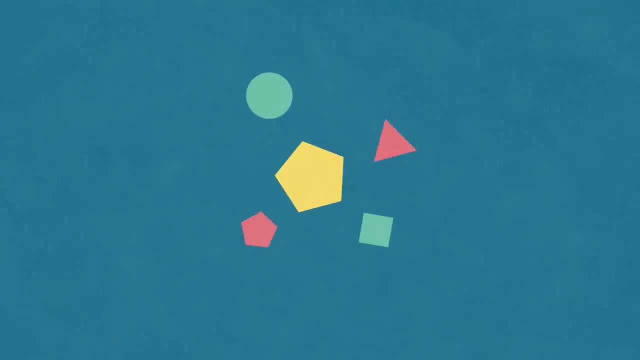 the guidelines of a good argument essay. The prize in this case was learning to write an argument essay, not learning to write about natural disasters. To differentiate by process, teachers can change up how they group students. Sometimes a mixed ability group might work best, while sometimes it might be appropriate to have 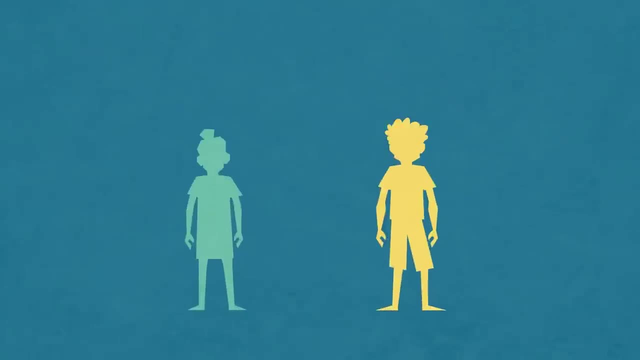 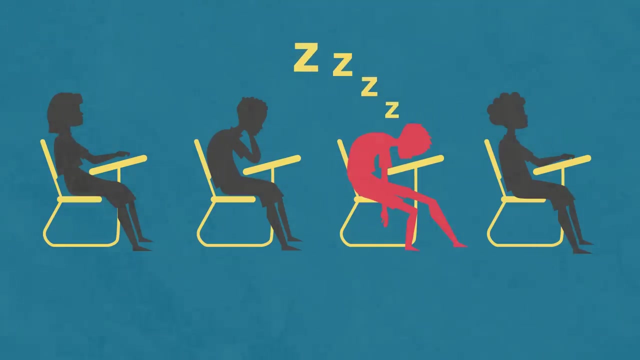 same ability groups. We might have an English proficient buddy work with an English language learner to help them out. During independent reading time in my early morning class several years ago, one student tended to fall asleep. I told him that if he wanted he could go to the. 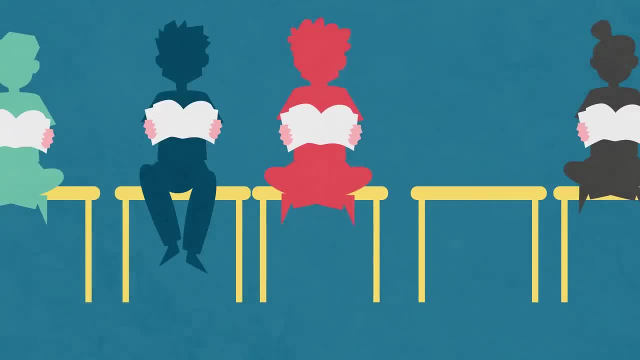 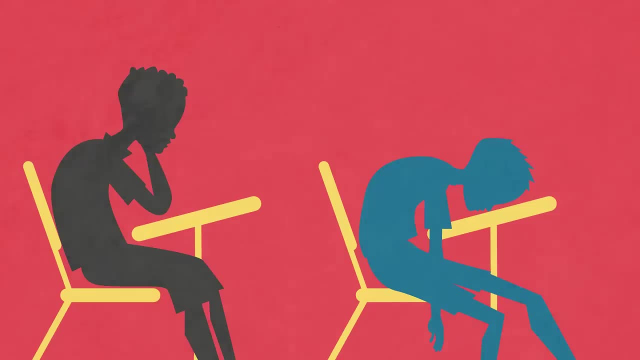 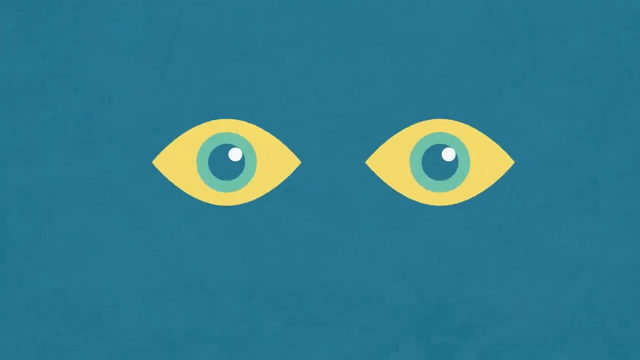 back and sit on a desk and read. Soon several others joined him. A few days later, I saw him dozing off. Before I could say anything, one of his classmates whispered to him: just go sit on a desk. Again, it's a matter of keeping our eyes on the prize. What are the? 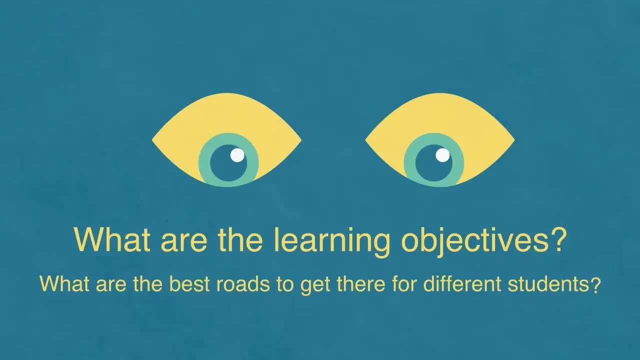 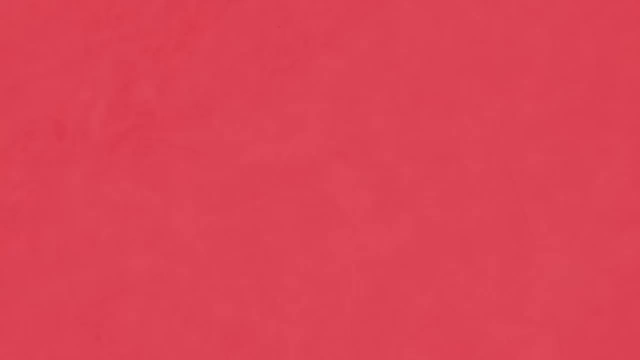 learning objectives and what are the best roads to get there for different students. Teachers can also differentiate by the type of product students create. The major demonstration of learning doesn't always have to be an essay or a multiple choice test. One year I had a student. 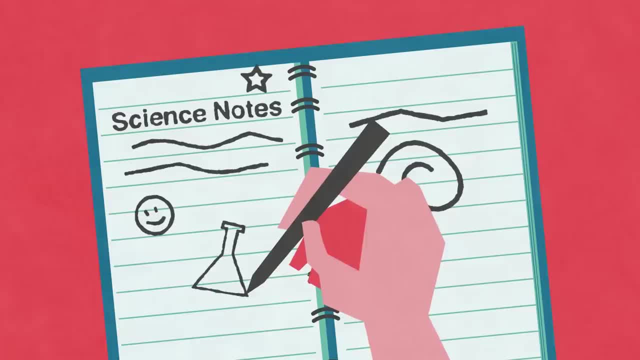 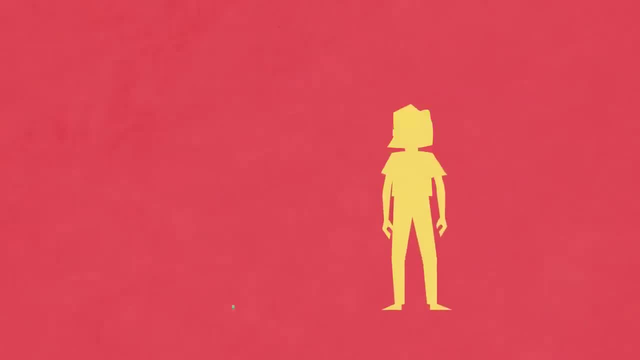 and a child in our class dino-doodle when other students or I were talking. I told her it was okay as long as she was doodling about the information we were discussing. She built on those doodles to create a final project that brilliantly and visually represented.